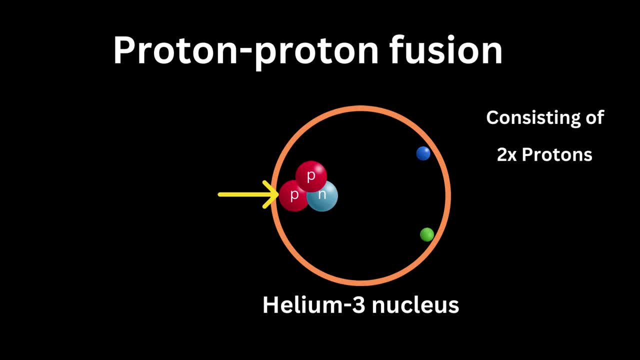 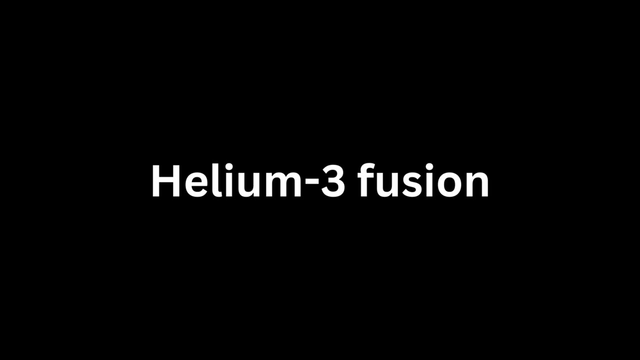 to create a helium-3 nucleus: two protons and one neutron. A gamma ray photon is released by this process. This brings us on to number 3. Helium-3 fusion. There are two possible routes for the helium-3 nucleus created in the step explained. These are path 1. Helium-3 fusion When two 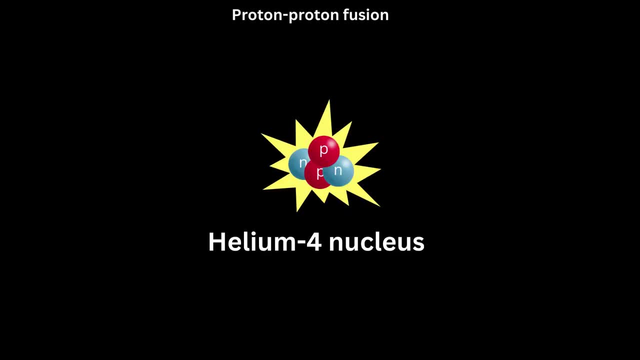 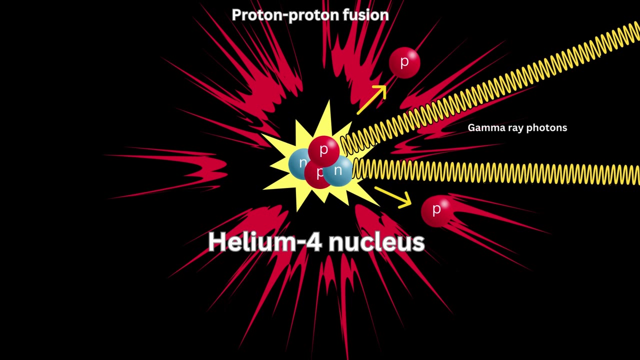 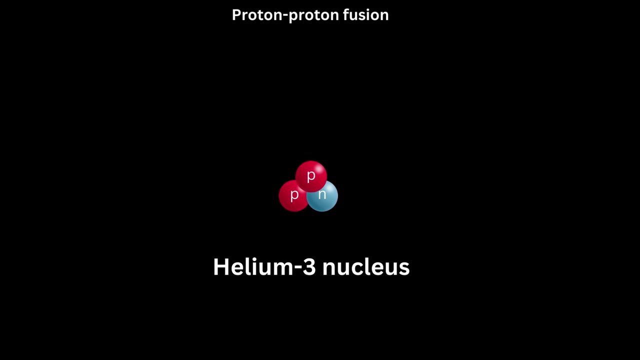 helium-3 nuclei collide, a helium-4 nucleus, which consists of two protons and two neutrons, are produced. Two protons, two gamma ray photons and a significant quantity of energy are released in this process. Path 2. Helium-3 capture: A helium-3 nucleus captures a helium-4 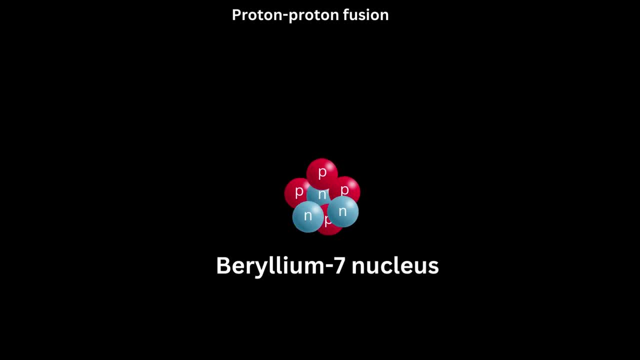 nucleus to create a beryllium-7 nucleus which consists of two protons and two neutrons. This route contains four protons and three neutrons. A gamma ray photon is released by this process. 4. Beryllium-7 decay, A lithium-7 nucleus which is three protons and four neutrons. 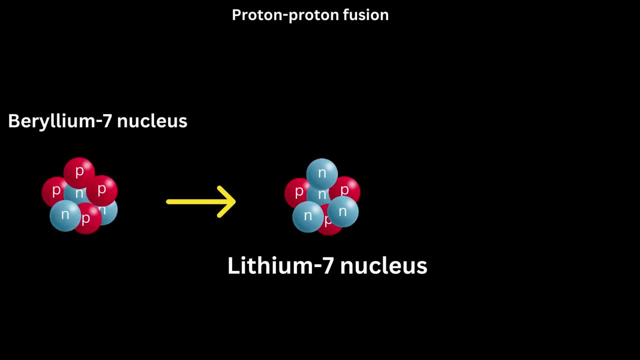 is created. when the beryllium-7 nucleus experiences beta-minus decay, An electron, an antineutrino, as well as some energy are released from the beryllium-7 nucleus. The lithium-7 nucleus does not directly take. 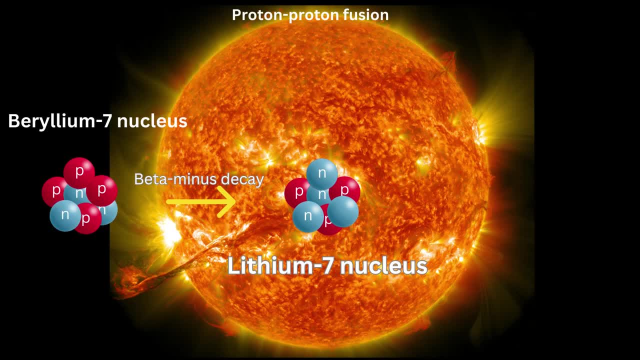 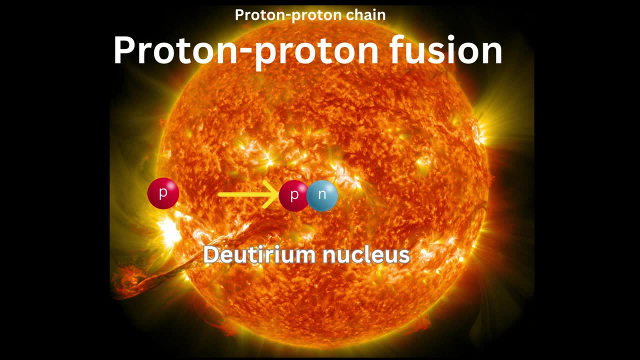 part in subsequent fusion processes within the sun after the beryllium-7 decay. As was mentioned in the earlier steps of the proton-proton chain, the primary reactions in the sun's core involve the fusion of protons to generate helium nuclei. 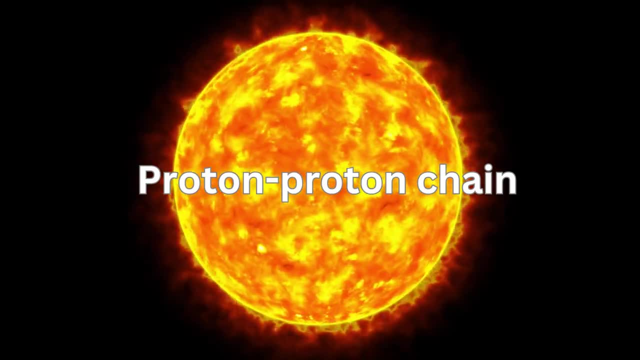 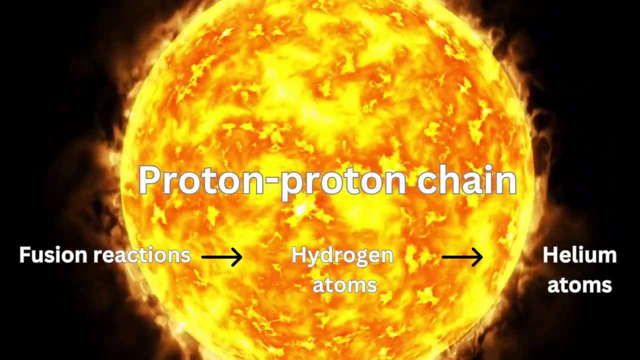 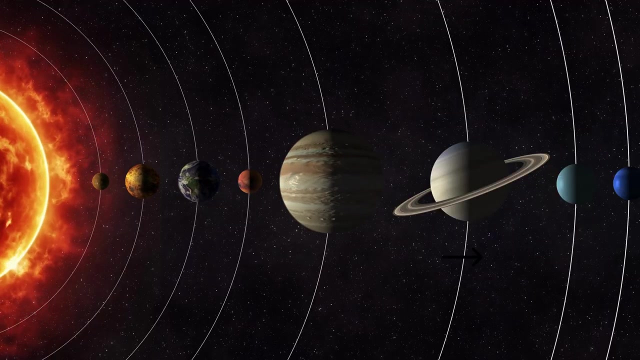 The proton-proton chain in its entirety consists of a succession of fusion reactions. These are the reactions that change hydrogen atoms into helium atoms, thus releasing energy in the form of gamma ray, photons and other particles. Our solar system receives heat and light from the sun thanks to this amazing energy.